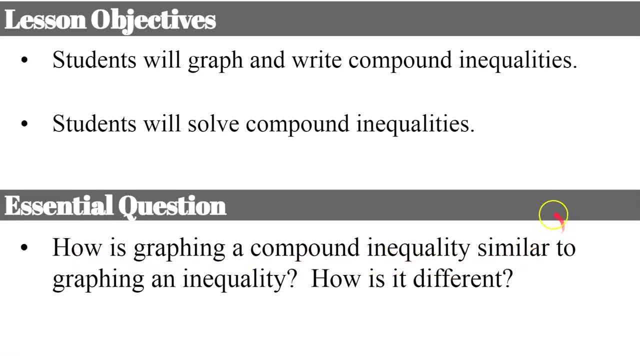 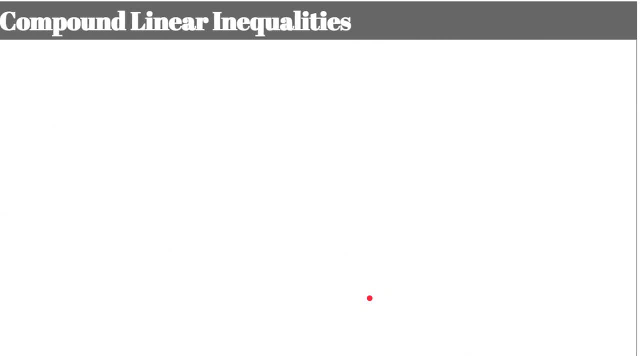 How is graphing a compound inequality similar to graphing an inequality And how is it different? Let's begin So. compound linear inequalities are inequalities formed by joining two inequalities, and they're either joined with the word and or with the word or 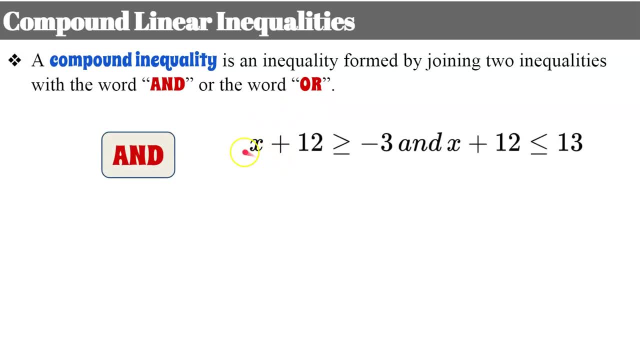 So we have and, and it would look like this, or it could look like this: We have an inequality that could stand alone, joined by and, and a second inequality: It could also, when it's an, and, be written in this fashion: 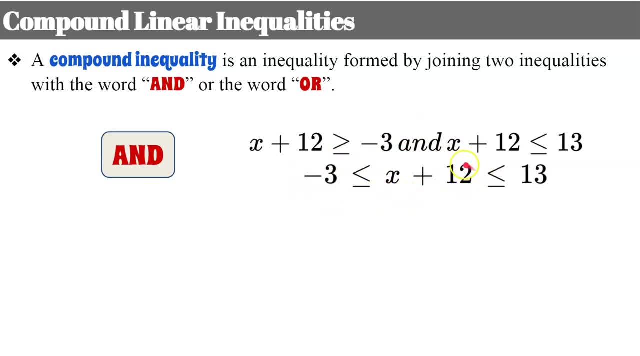 So think of it as right here we have negative 3 less than or equal to x plus 12, and our second inequality is right here: x plus 12 is less than or equal to 13.. So there are two inequalities that can be split into two inequalities that look like this: 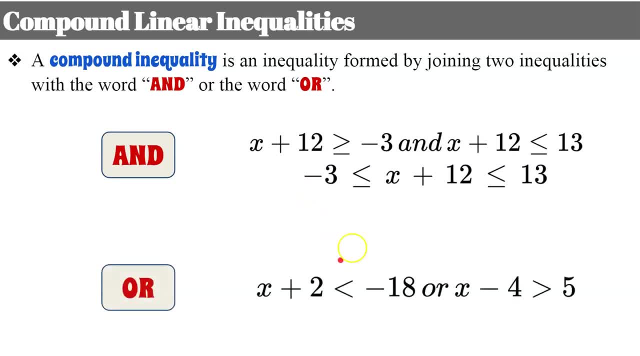 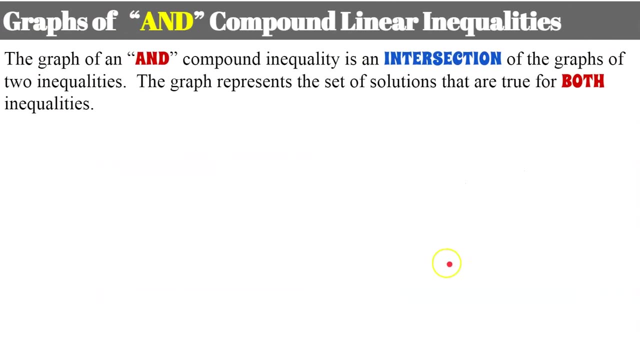 When you have an or, it will look like this. There's no way to write it a second way: It has to be two inequalities. It has to be joined by the word or, So I have a standalone inequality or this inequality. Graphs of the and compound inequalities are an intersection of the graphs of the two inequalities. 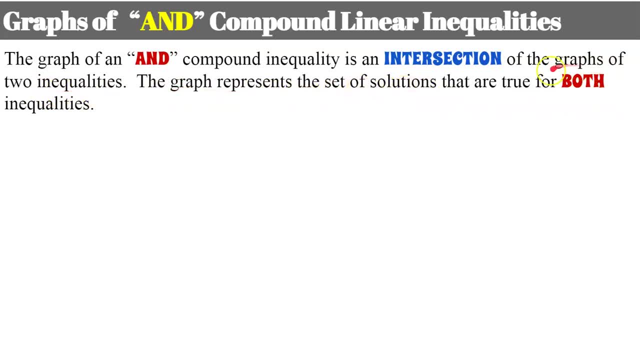 The graph represents the set of solutions that are true for both inequalities. So think about joining what the overlap is and that is your solution set. So let's look at one. So I have a simple compound: inequality. This is what your solutions will look like once you've solved a compound and inequality. 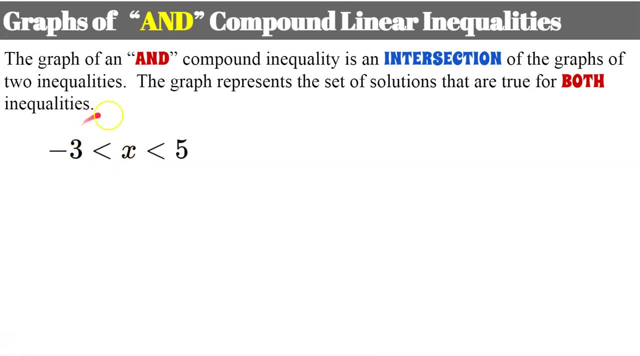 So really this says x is greater than negative 3, and x is less than 5.. So remember when you reverse where the variable is if you flip it to the other side. so right now it's on the right of the inequality symbol. 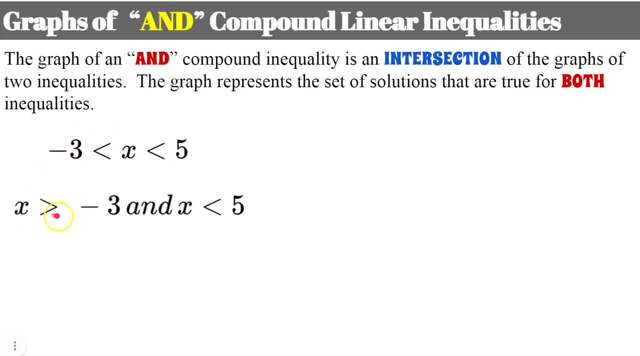 If I flip it so that it's on the left, I must also flip the inequality symbol. And when there's no inequality, I must also flip the inequality symbol. And when there's no words and it's written like this, we know that the word is and. 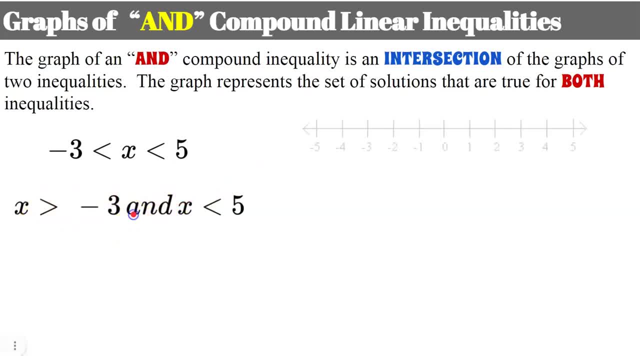 So let's think about graphing it First. I'm going to graph this inequality, So here's my two number lines. So we're going to have an open circle on negative 3, because it's greater than but not equal to, And because it's greater than, my arrow is going to go to the right. 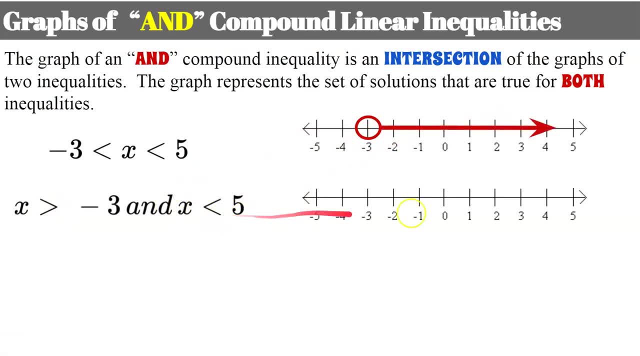 The second inequality is going to have an open circle because it's not equal to on 5, and it's less than So. notice that these are all the values Greater than, and here it's less than So. this intersection, right here is our solution set. 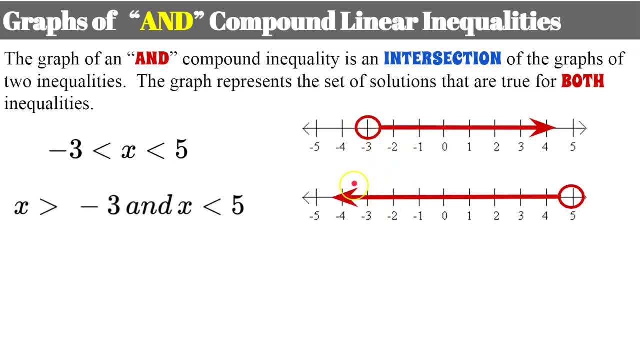 So you would not graph this compound inequality like this. I just did this to show you how you graph them individually. So if we're going to graph this solution set, it's going to begin with an open circle at negative 3,, stop with an open circle at 5, and we're going to shade everything in between. 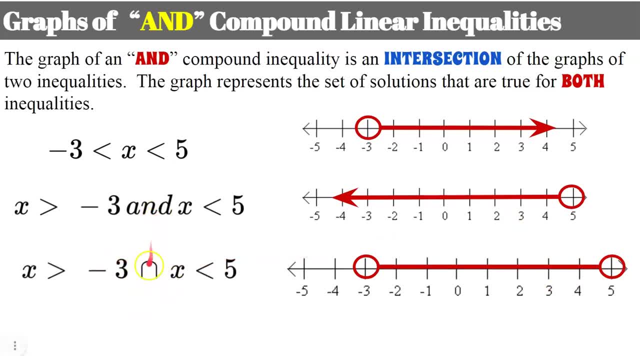 So I'm going to take away- we can call this the intersection, That's another way to write it- So the intersection of these two solution sets, and this is the symbol for intersection in math. So right here, this graph shows the intersection of this solution set and this solution set. 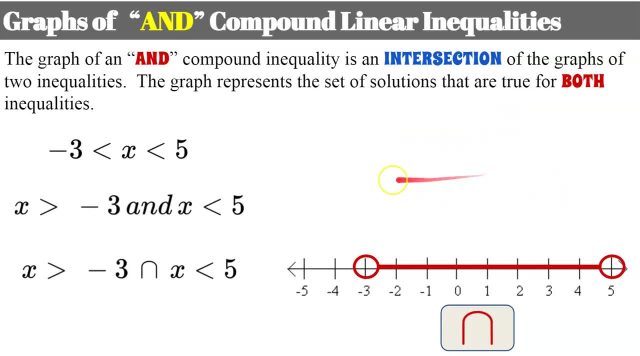 So we're going to take away these graphs. okay, because those aren't true for this compound inequality. They were true for individual inequalities. So when we look at the solution set for this- and this is what it's going to look like- 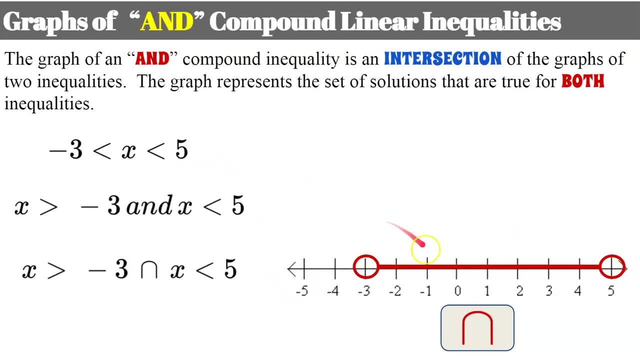 Okay. So whenever you see or have a compound inequality with the word and it's an intersection of the two solution sets, So it's not all the solutions of x is greater than negative 3, or all the solutions of x that's less than 5.. 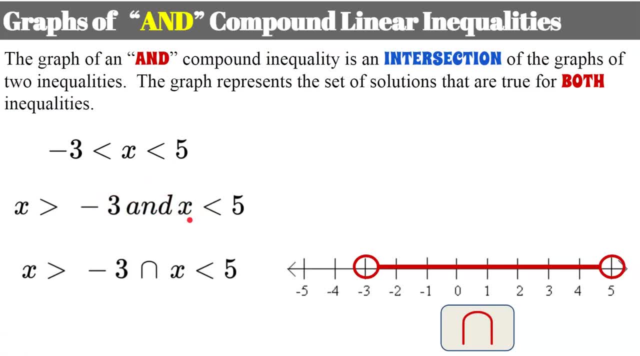 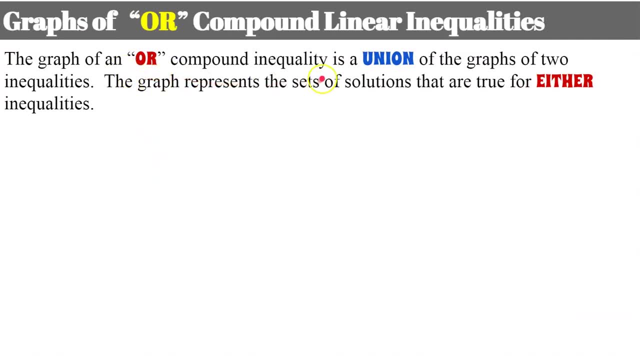 It's the solutions that are true for both inequalities. Now let's talk about the graphs of the or compound inequalities. The graph of an or compound inequality is the union of the graphs of the two inequalities. The graph represents the sets of solutions that are truth for either inequalities. 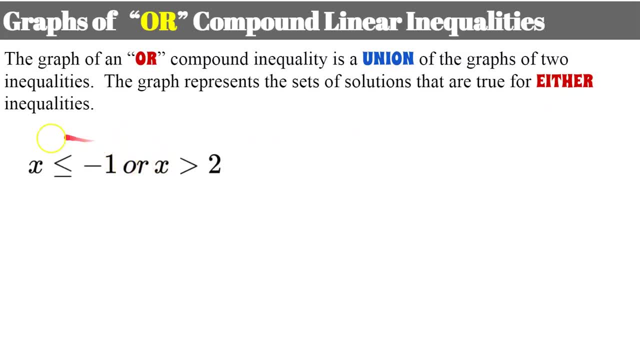 So here, when you have an, or you always see the word, or We have the inequality: x is less than or equal to negative 1, or x is greater than 2.. So we're going to put, combine, make a union of the two solution sets. 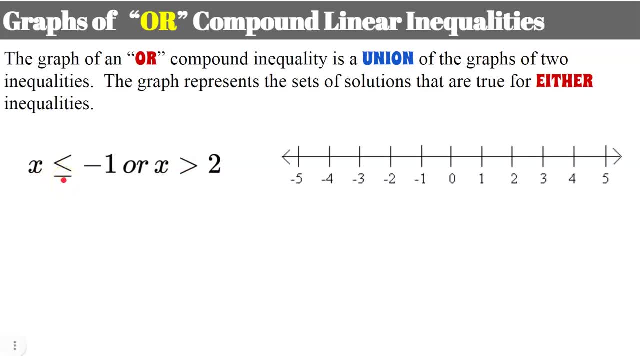 So on our number line, the first thing I want to do is put a solid or a closed circle on negative 1, because it can be equal to. So negative 1, closed circle And or All the solutions less than, And then open circle because it's greater but not equal to. 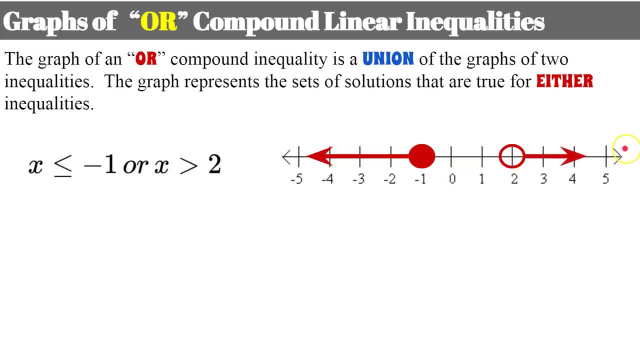 So our solution set for this one goes to the left and our solution set for that one goes to the right, And we can write this as the union. So there's no intersecting, there's no overlapping. So a true solution for this compound inequality is anything found from negative 1 less. 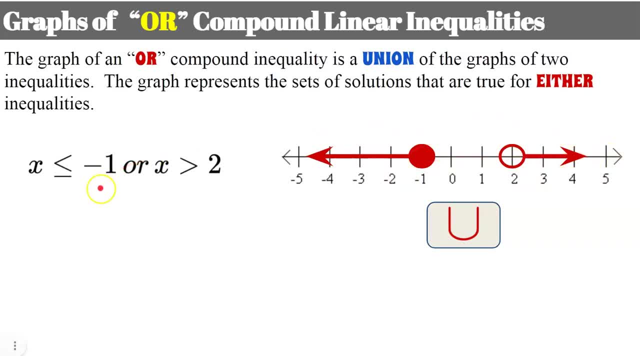 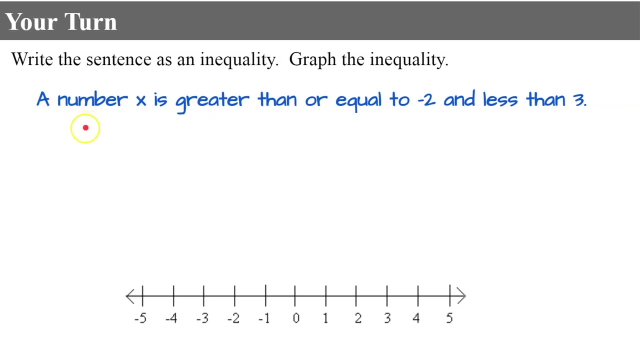 or greater than 2.. Either one of those is a solution to this compound inequality, So we could Also replace the or with this symbol for union. All right, your turn. I would like you to write the sentence written in blue: A number x is greater than or equal to negative 2 and less than 3.. 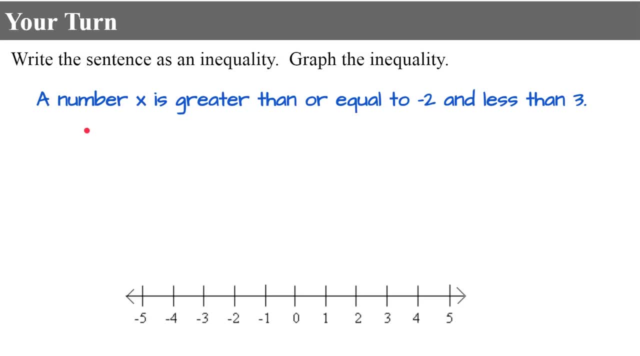 And then I would like you to graph the inequality that you write. Please pause and come back when you're ready. Welcome back. So our solution first is our number x. Let's highlight: we have a number x greater than or equal to negative. 2 is our first inequality. 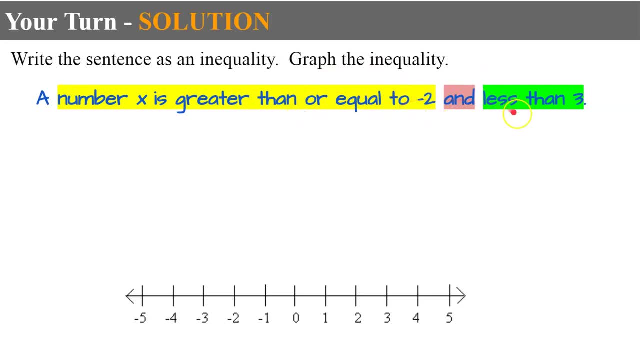 It's an and compound inequality, And our second is going to be a number x less than 3.. So we have a number x greater than or equal to negative 2. And a number x less than 3.. So now, when we go to graph it, we're going to graph a closed circle on negative 2.. 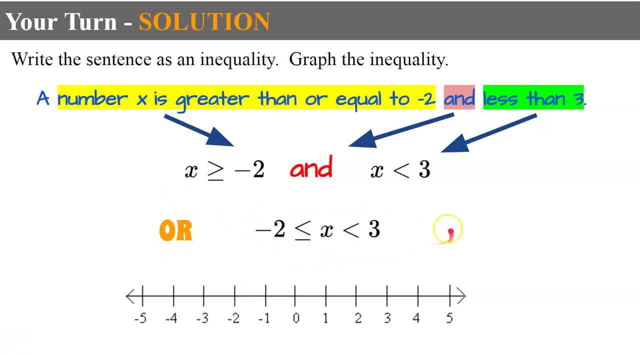 Or we could write it like this too- I forgot that part, So we can take the and out. we're flipping this, so we have to reverse the symbol. So because I'm moving the negative 2 to the left, I have to reverse the inequality symbol. 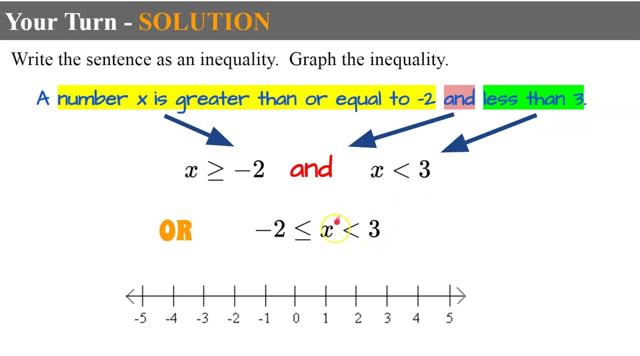 Our x goes in the middle and our less than 3.. So be careful when you write it like this, And I always. as a general rule of thumb, the number on the far left is the number that's the least in value. Now let's graph. 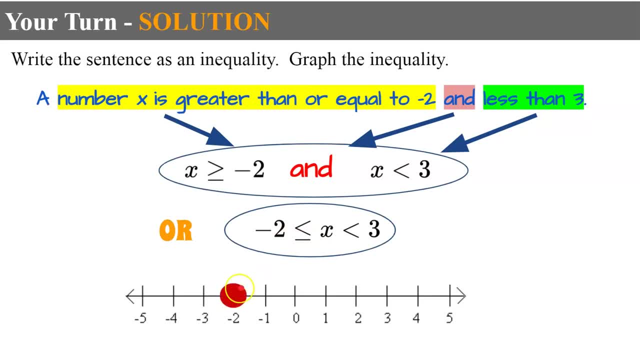 So we're going to have a closed circle on negative 2. And shaded to the right because it's greater than or equal to, Open circle on 3 because it cannot be equal to it And everything less than So. our graph is the solutions of negative 2 all the way up until the value of 3.. 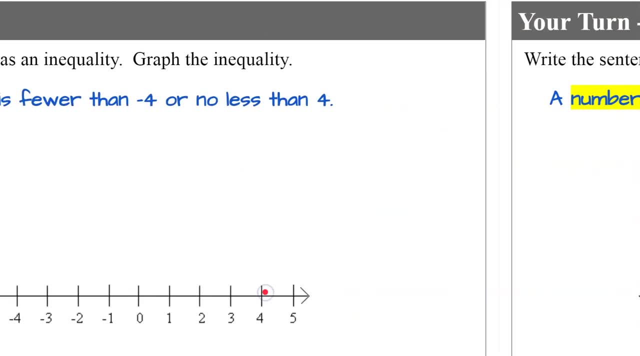 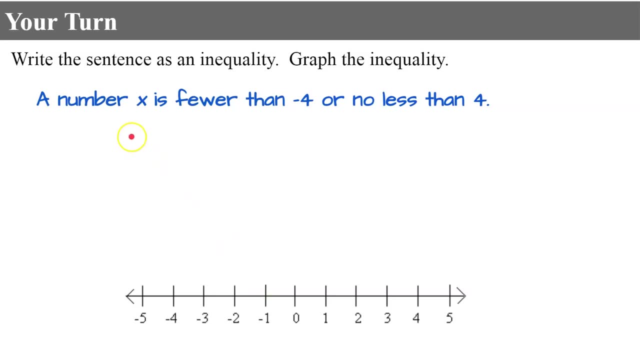 The intersection of the two graphs. Your turn, Let's try this one. I would like you to write the sentence below in blue as an inequality and graph it. A number x is fewer Than negative, 4 or no less than 4.. 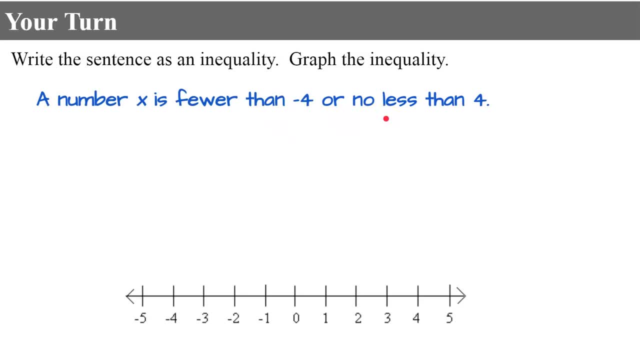 Please pause now and come back when you're ready. Welcome back. So we first want to identify that we have our first inequality- It's a compound or inequality- and then a number- x no less than 4.. So a number fewer than 4 is going to be less than is fewer than is the same as saying less than negative 4.. 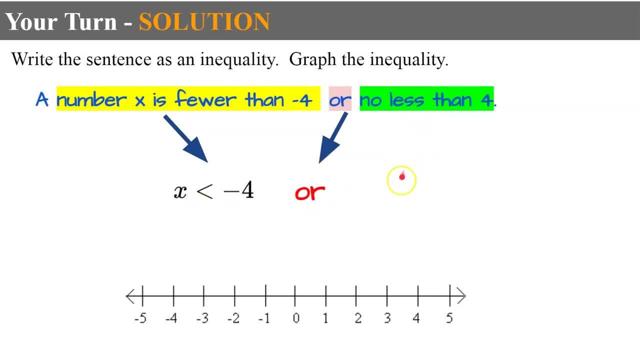 We have our or. And then We have a number x no less than 4. So it has to be greater than or equal to 4.. So it can be 4, but it can't be less than 4 on this one. 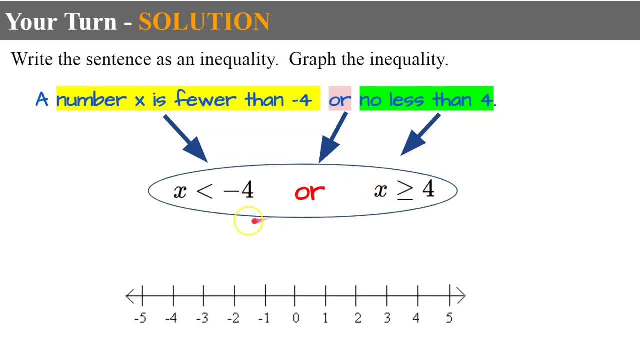 So when we go ahead- there's no other way to write this- We're going to graph. we're going to graph an open circle on negative 4 because it's not equal to And it's all the values less than that. Then we come over here. we're going to have an open circle on 4 because it can be equal to 4.. 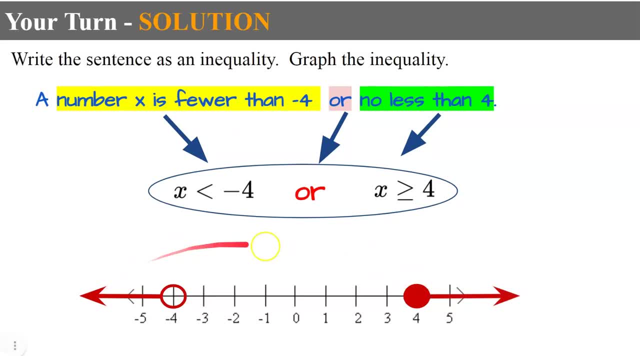 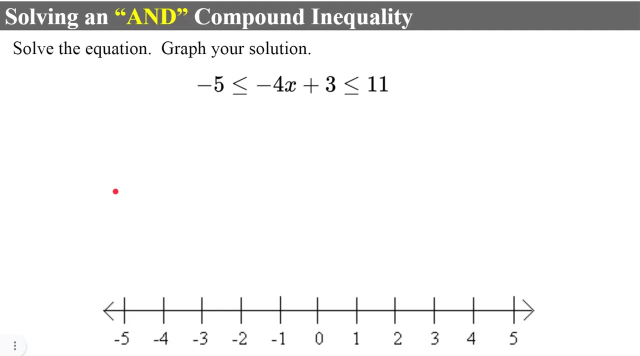 And then all the solutions to the right. So we call this a union, because nothing intersects. So it's all the solutions here or all the solutions here. If it falls in either, then it's true for this compound inequality. Now let's talk about solving an and compound inequality. 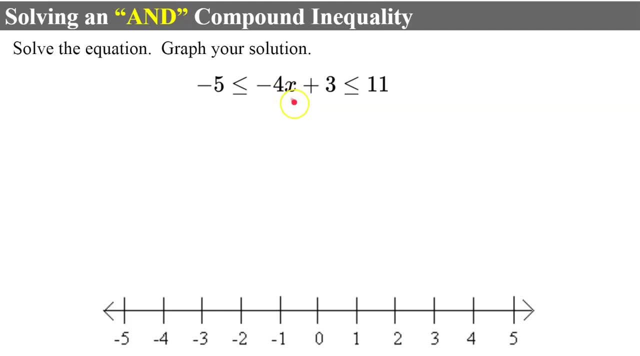 So we're going to solve this and graph our solution. So the first thing I'm going to do is recognize that this is an and and it can be split into two inequalities. So I have the negative 5 less than or equal to negative 4x plus 3.. 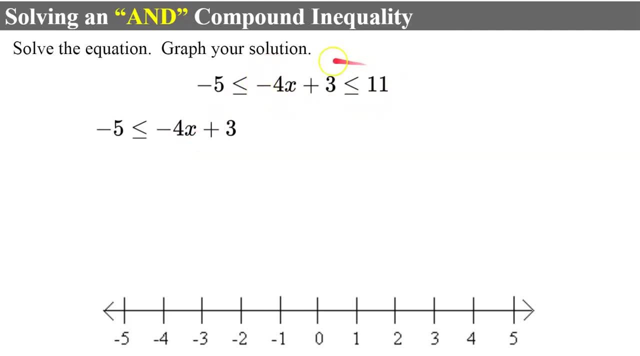 It's my first, and my second is going to be negative 4x plus 3 less than or equal to 11.. Now I'm going to solve these separately. So the first thing I'm going to do is isolate the variable term by doing the inverse of add 3, which is to subtract 3 from both sides. 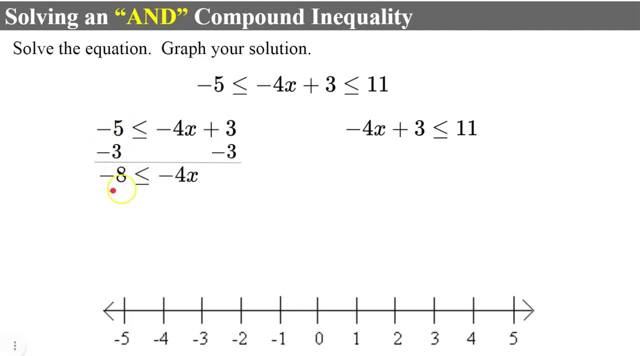 Leaving me negative 8, negative 5 and negative 3, or negative 8 less than or equal to negative 4x. Now I want to isolate the x, so I'm going to do the inverse of multiply by negative 4.. And divide both sides by negative 4.. 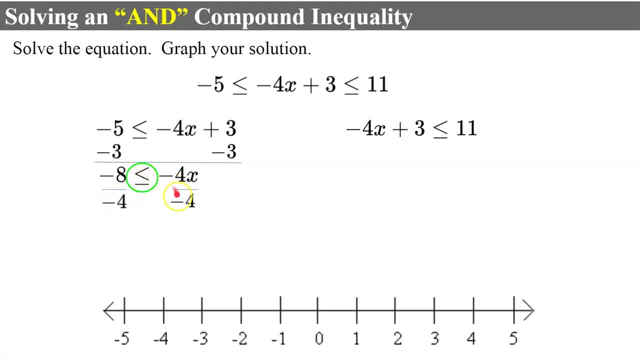 And flip my sign. I got to reverse the direction of the sign because I'm dividing by a negative value: Negative 8 divided by negative 4 is a positive 2. I reverse the direction of my symbol and I have x. So now we're going to solve the second inequality. 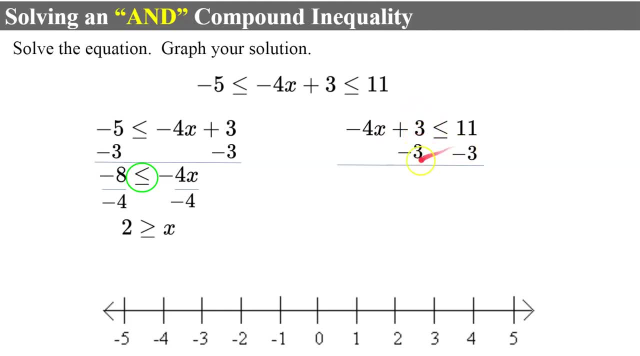 I'm going to do the inverse of add 3, and that is to subtract 3 to both sides, Leaving me negative 4x, and 11 minus 3 is 8.. Now I'm going to divide both sides by the coefficient of negative 4.. 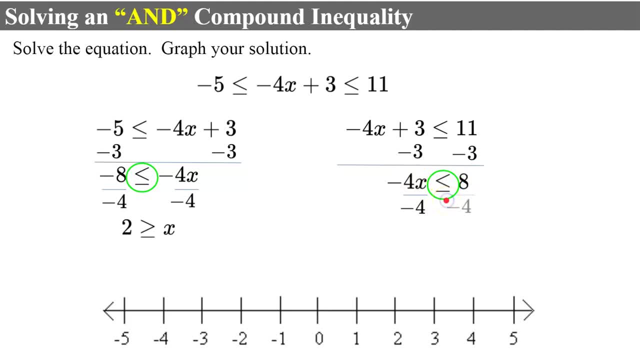 Knowing that I'm dividing by a negative value and I have to reverse the direction of the symbol That leaves me x Flip my sign Greater than or equal to negative. 2. Remembering that, the way this is written, it's an. and. 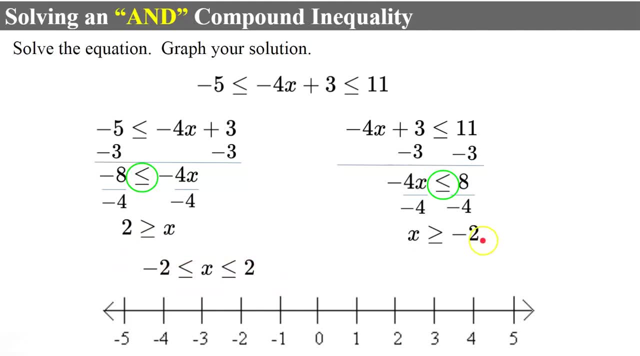 So you could combine them like this: Negative 2. I always start with the less value, Negative 2. I'm flipping it, So I'm going to reverse the direction of the symbol x Again. I'm flipping this one too. 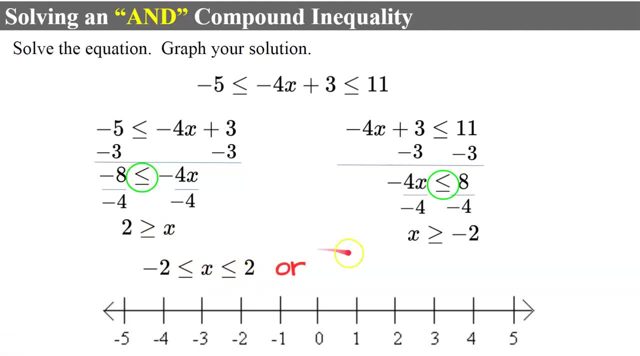 So I'm reversing my symbol 2.. Or I could say: x is greater than or equal to negative 2 and x is less than or equal to 2.. So let's graph these. I'm going to graph this one first. I'm going to put a solid circle on negative 2.. 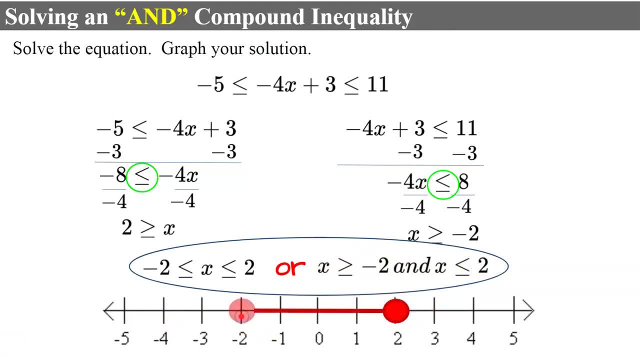 Solid circle on 2 was first, And then a solid circle on negative 2 and shade everything in between. So it's an intersection Off, or larger than or equal to 2.. Now we're gonna solve an or inequality. So you can see I have one inequality. 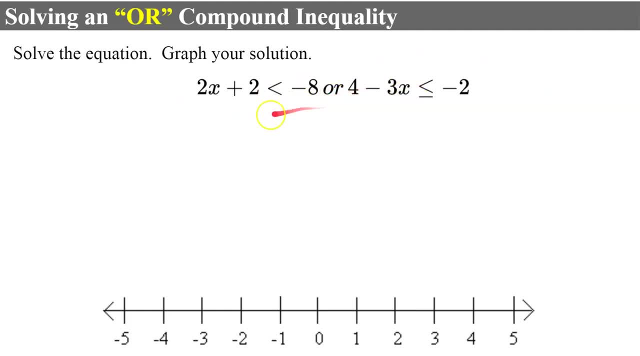 Or and then a second inequality. So we're gonna solve these two inequalities separately. The first thing I'm going to do here is I'm writing 2 down. I'm going to do the inverse of add 2 and subtract 2 from each side. 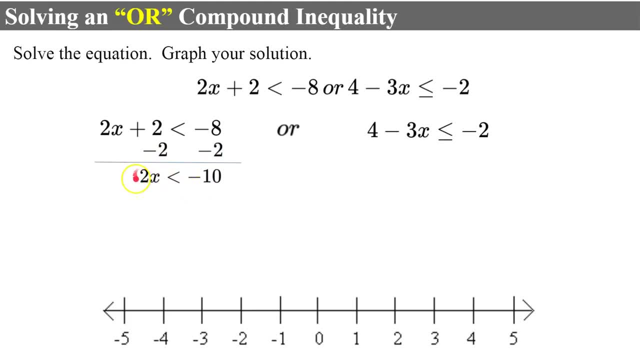 Giving me 2x is less than negative 10.. Divide both sides by 2.. It's a positive, so I do not reverse the symbol. So I do name the 4 and 9 times And I got x-2.. I'm going to write 2 down. I'm not going to revert these. 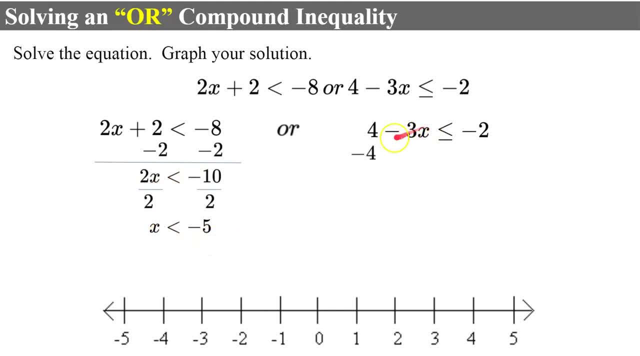 x is less than negative 5. and then I'm gonna come up and I'm gonna subtract 4 from both sides, leaving me negative 3x is less than or equal to negative 6. divide both sides by negative 3 and reverse the direction of my symbol. 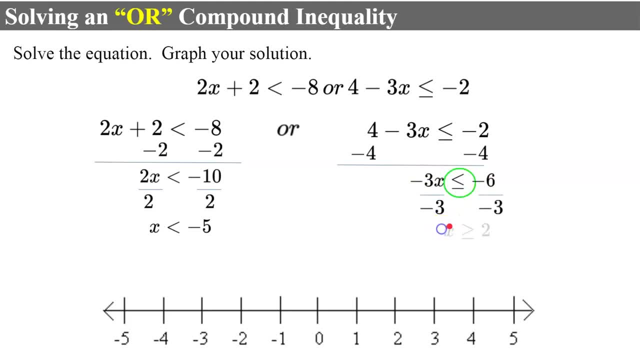 because I'm dividing by a negative value x greater than or equal to 2, remembering that this is an OR, so I have to graph: x is less than negative. 5. open circle arrow to the left. closed circle because it can be equal to and greater than that shaded to the right. so this is a union. anything in this solution set or: 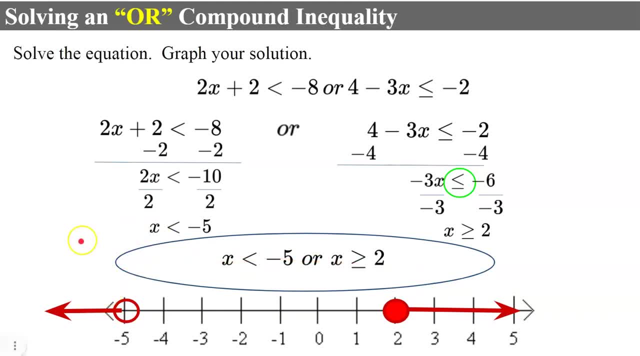 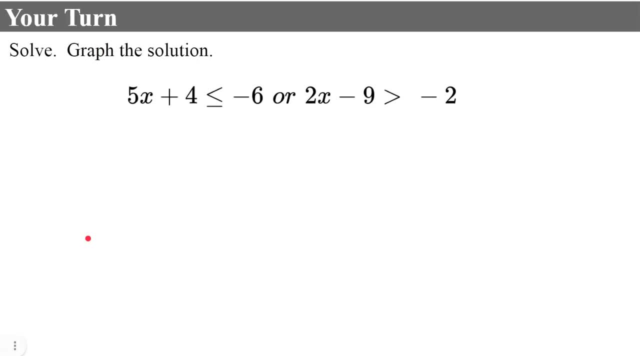 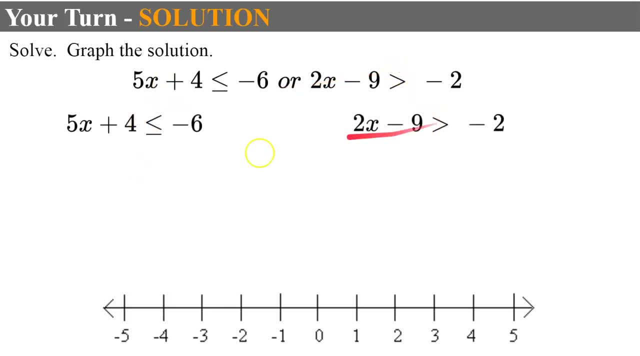 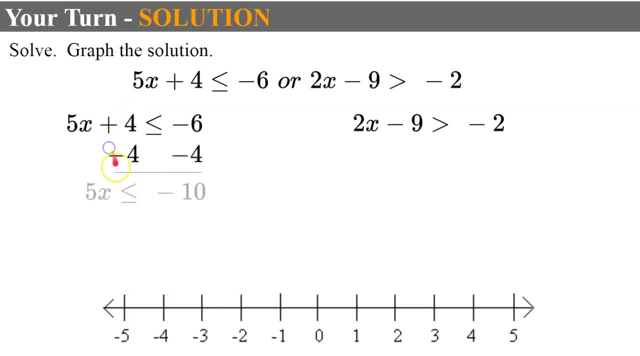 the second. so I'm gonna isolate the variable term by subtracting 4 from each variable term. by subtracting 4 from each variable term. by subtracting 4 from each side, leaving me 5x is less than or side, leaving me 5x is less than or. 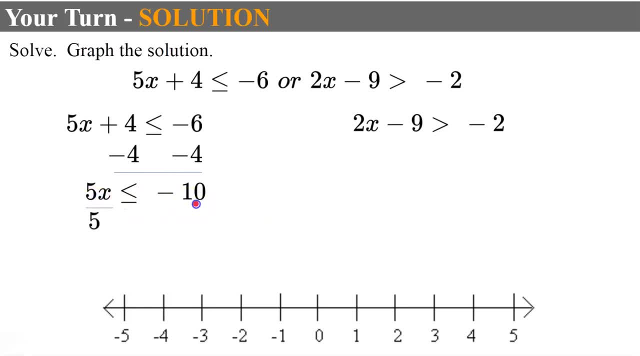 side, leaving me 5x is less than or equal to negative 10. divide both sides by 5: equal to negative 10. divide both sides by 5: equal to negative 10. divide both sides by 5. it's a positive value, so I will not. 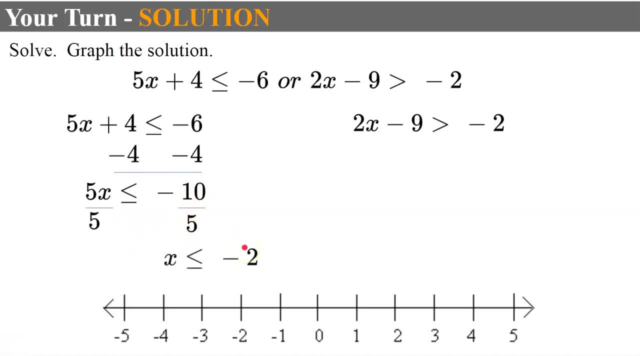 it's a positive value, so I will not. it's a positive value, so I will not. reverse the symbol. and negative 10: reverse the symbol and negative 10: reverse the symbol. and negative 10 divided by 5 is negative 2, then I have my. 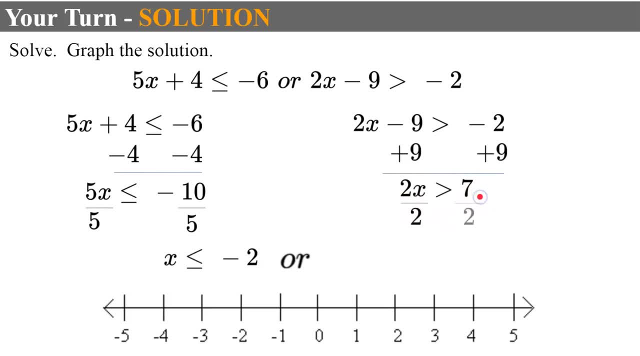 divided by 5 is negative 2, then I have my. divided by 5 is negative 2, then I have my 7. divide both sides by 2. I do not need 7. divide both sides by 2. I do not need 7. divide both sides by 2. I do not need to reverse the symbol because I'm 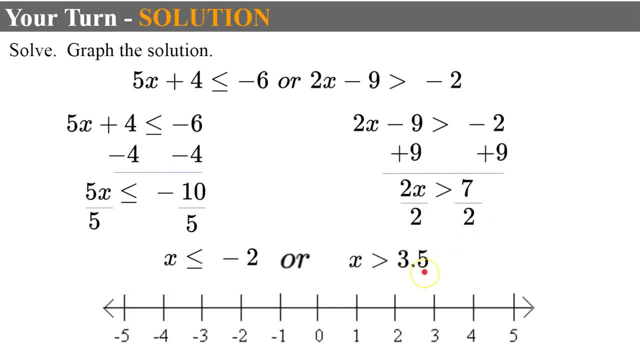 to reverse the symbol. because I'm to reverse the symbol? because I'm dividing by a positive, so X is greater. dividing by a positive, so X is greater. dividing by a positive, so X is greater than 3.5. let's graph: so we're gonna have: 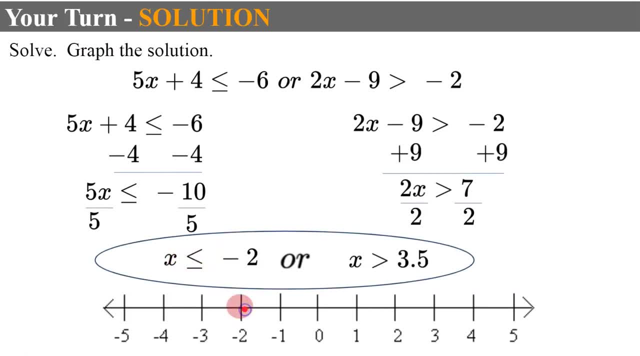 than 3.5. let's graph so we're gonna have than 3.5. let's graph so we're gonna have a solid circle on negative 2. because it a solid circle on negative 2. because it a solid circle on negative 2 because it can be equal to and shaded to the left. 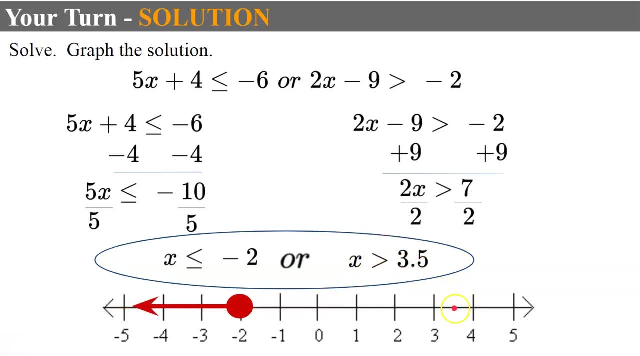 can be equal to and shaded to the left, can be equal to and shaded to the left. an open circle on 3.5, because it cannot. an open circle on 3.5, because it cannot. an open circle on 3.5, because it cannot be equal to and then greater than so. 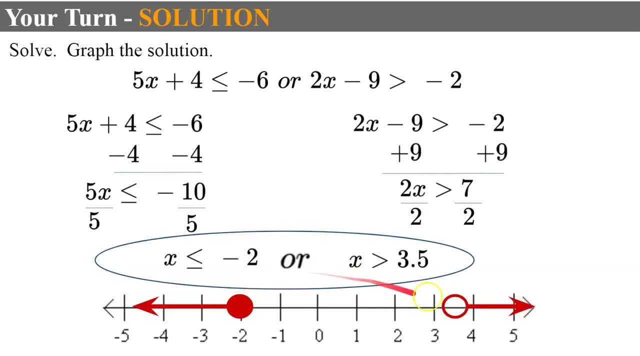 be equal to and then greater than so. be equal to and then greater than so. shaded to the right. so again, this is a shaded to the right. so again, this is a shaded to the right. so again, this is a union, because it's anything in this union, because it's anything in this. 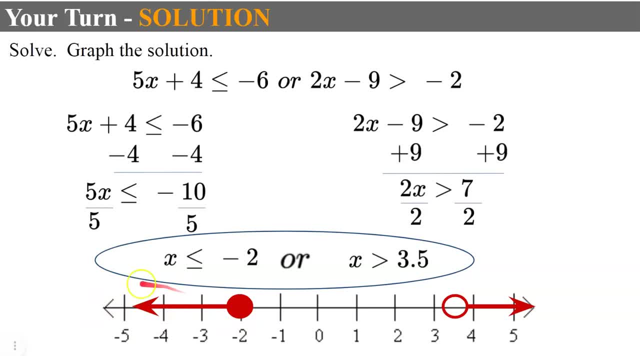 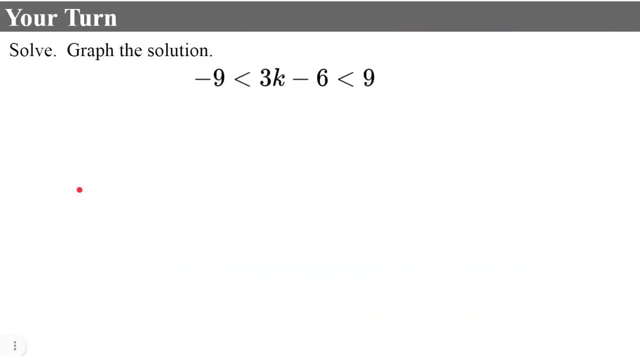 union, because it's anything in this solution set or anything in this solution set or anything in this solution set or anything in this solution set is a solution to the solution set is a solution to the solution set is a solution to the compound inequality. your turn, go ahead. 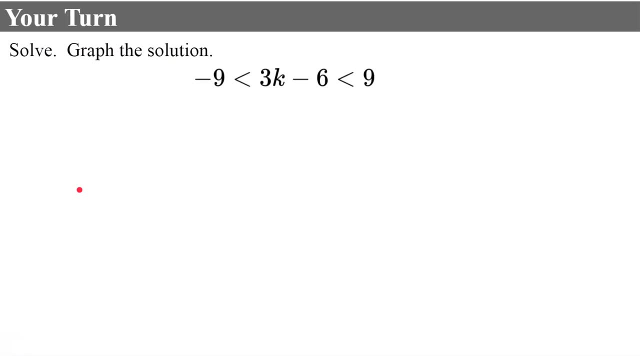 compound inequality. your turn, go ahead. compound inequality, your turn, go ahead and solve graph and come back to check and solve graph. and come back to check and solve graph and come back to check your work, welcome back. so the first thing: your work, welcome back. so the first thing I want to do is this is an: and so 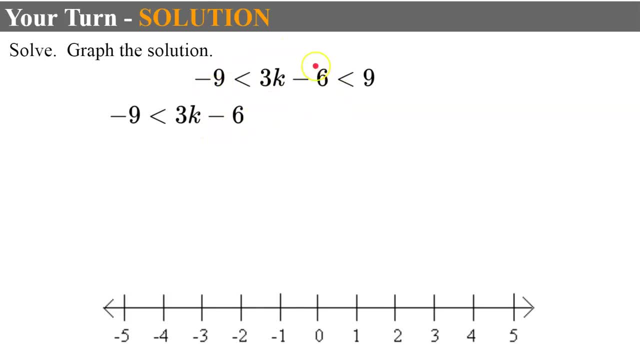 I want to do is. this is an, and so I want to do is. this is an, and so we're going to separate. we have negative 9: we're going to separate. we have negative 9: we're going to separate. we have negative 9. less than 3 K plus 6 is my first. 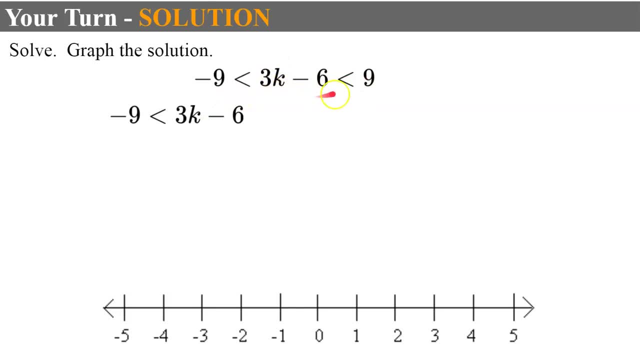 less than 3 K plus 6 is my first. less than 3 K plus 6 is my first inequality. my second inequality is going inequality. my second inequality is going inequality. my second inequality is going to be 3 K minus 6. less than 9 separated. 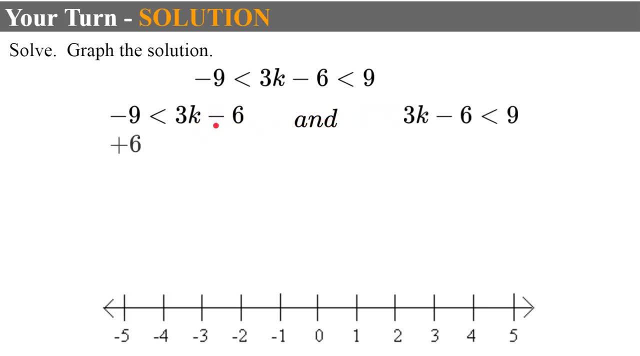 to be 3 K minus 6, less than 9 separated. to be 3 K minus 6, less than 9, separated by. and so let's solve our first. we're by, and so let's solve our first. we're by, and so let's solve our first. we're going to add 6 to each solid, giving me 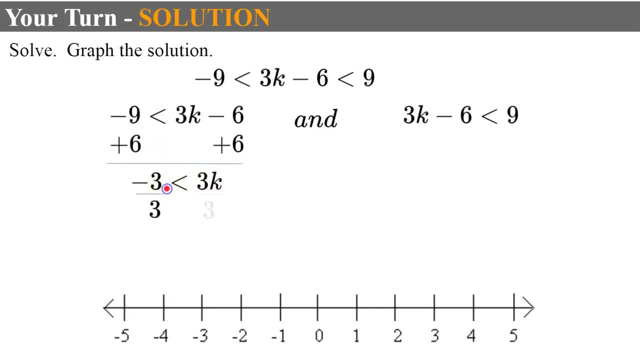 going to add 6 to each solid, giving me going to add 6 to each solid, giving me 3 K less than negative. 3. divide both 3 K less than negative. 3. divide both 3 K less than negative. 3. divide both sides by 3 for a solution of negative 1. 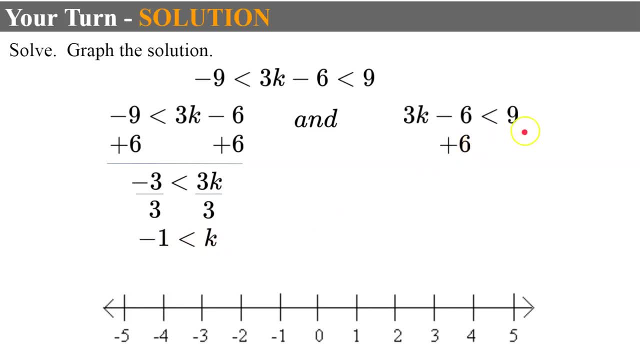 sides by 3 for a solution of negative 1. sides by 3 for a solution of negative 1 less than K. add 6 to both sides. 3 K is less than K. add 6 to both sides. 3 K is less than K. add 6 to both sides. 3 K is less than 15. divide both sides by 3 and. 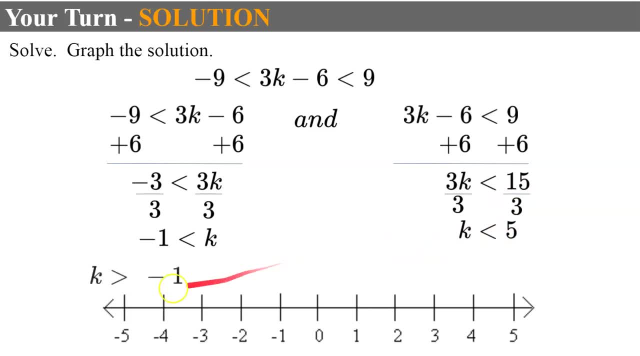 less than 15. divide both sides by 3. and less than 15, divide both sides by 3. and K is less than 5. and remember we could. K is less than 5 and remember we could. K is less than 5 and remember we could write. K is greater than negative 1. I. 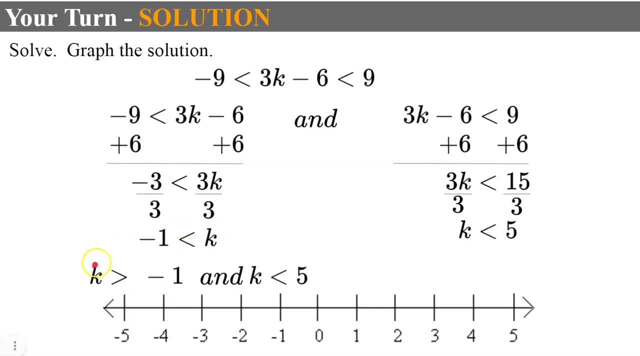 write K is greater than negative 1. I write K is greater than negative 1. I reversed where the K was, instead of reversed where the K was, instead of reversed where the K was. instead of putting it on the right, I put it on the. putting it on the right, I put it on the. 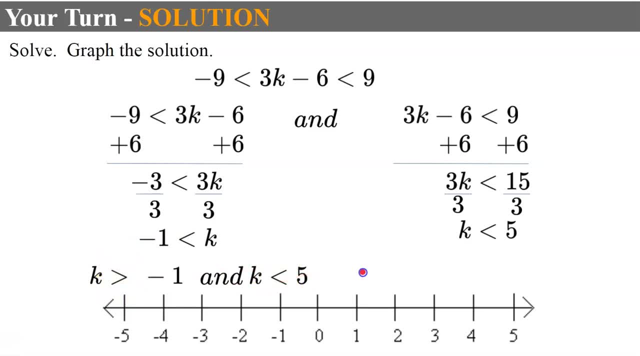 putting it on the right, I put it on the left, so I had to reverse my symbol and K left, so I had to reverse my symbol and K left, so I had to reverse my symbol. and K is less than 5 or I could write it in. 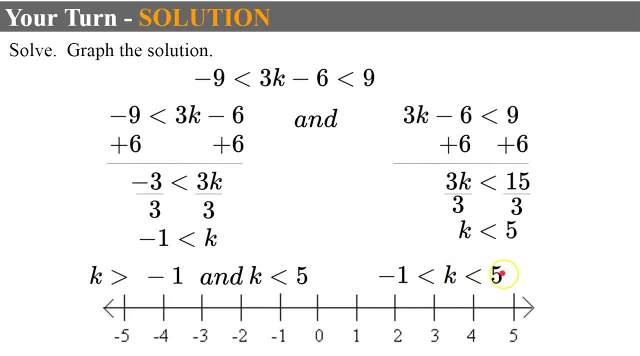 is less than 5, or I could write it in: is less than 5, or I could write it in this way: negative 1 less than K- less. this way: negative 1 less than K less. this way: negative 1 less than K less than 5. so let's go ahead and graph. 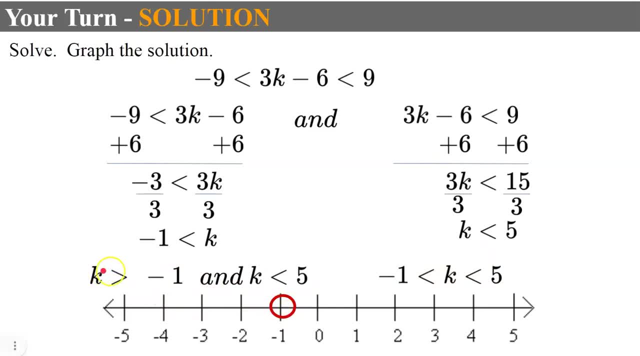 than 5. so let's go ahead and graph than 5. so let's go ahead and graph. we're going to have an open circle on. we're going to have an open circle on. we're going to have an open circle on negative 1 and it's all the solutions. 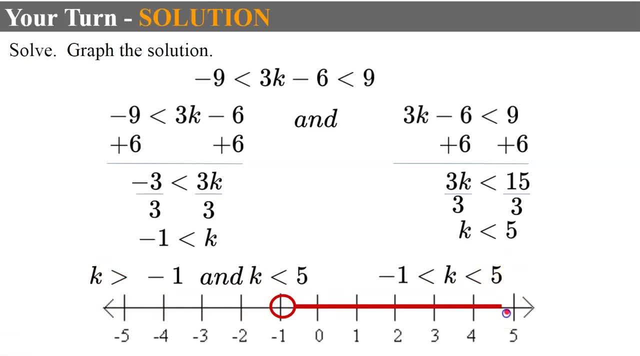 negative 1, and it's all the solutions. negative 1 and it's all the solutions. greater than that, and then an open greater than that, and then an open greater than that, and then an open circle on 5, because it cannot be equal. circle on 5, because it cannot be equal. 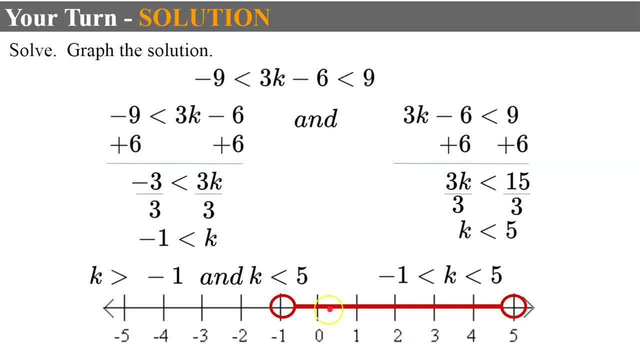 circle on 5, because it cannot be equal to, and all the solutions less than that to, and all the solutions less than that to, and all the solutions less than that. so this is an intersection. so the. so this is an intersection, so the. so this is an intersection, so the solutions that are true for this.